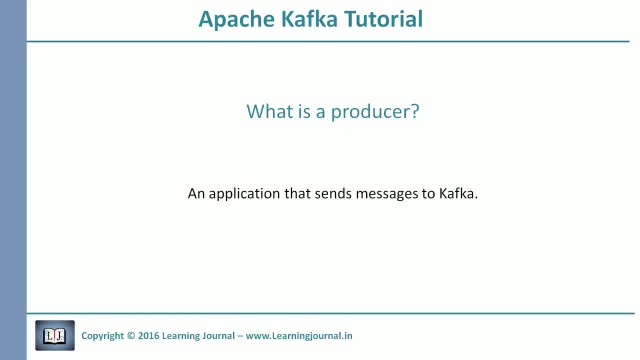 that sends data. Some people call it data, but we will call it a message. Ultimately, it is a small to medium-sized piece of data. The message may have different meaning or schema for us, but for Kafka it is a simple array of bytes. For example, if 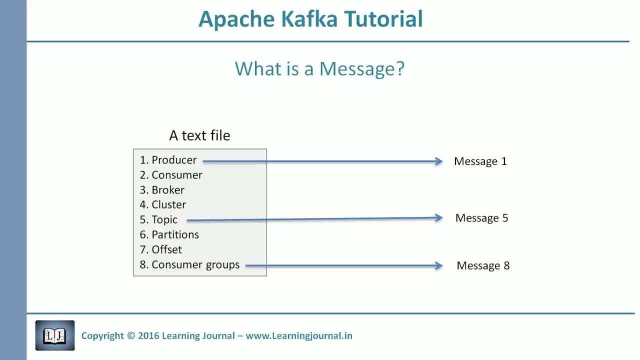 I want to send a file to Kafka. I will create a producer application and send each line of the file as a message. In this case, a message is one line of text, But for Kafka it is just an array of bytes. Similarly, if I want to send all the records, 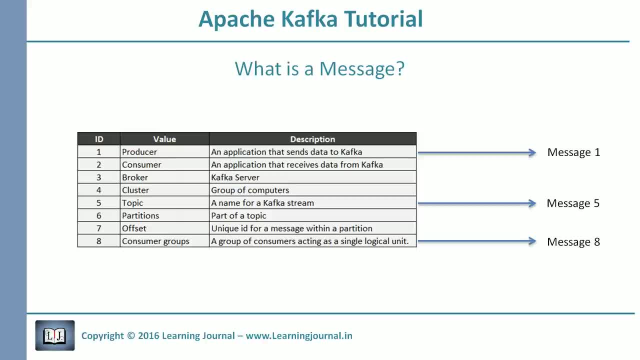 from a table, I will send each row as a message. Or if I want to send a result of a query, I will create a producer application, fire a query against my database, collect the result and start sending each row as a message. 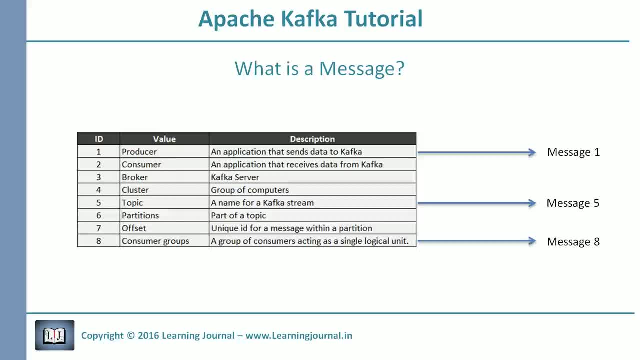 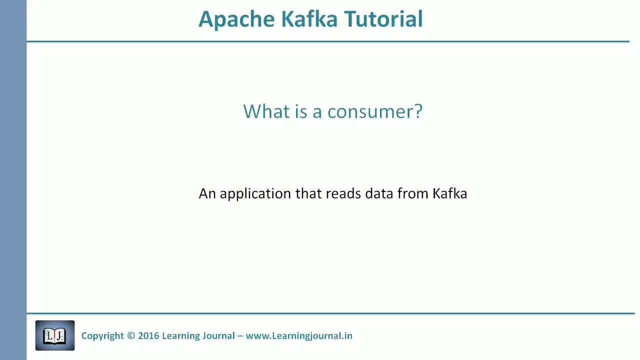 Kafka, if you want to send some data, you have to create a producer application. It is very unlikely that you get a ready-made producer that fits your purpose. I hope I am clear in explaining a producer and a message. The next thing is the consumer. So the consumer is again an application that receives data. 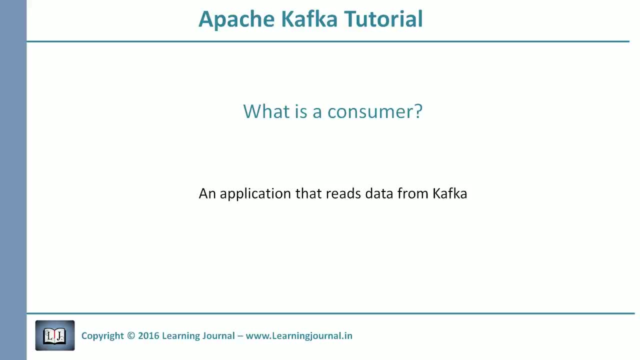 If producers are sending data, they must be sending it to someone right? The consumer is the application that receives data. Consumers are the recipient. But remember that the producer don't send data to a recipient address. They just send it to Kafka's server And anyone who is interested in that data. 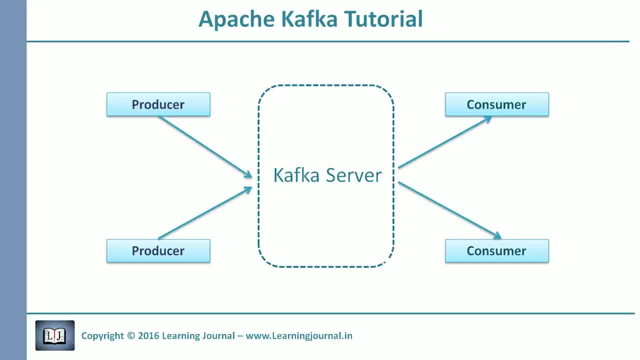 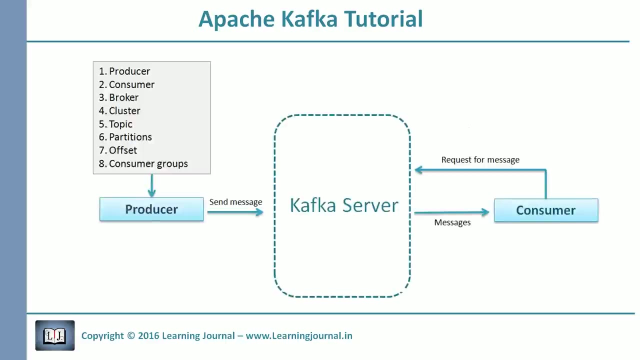 can come forward and take it from Kafka's server. So an application that requests data from a Kafka server is a consumer, And they can request for data sent by any producer, provided they have permissions to receive it. So the consumer is the recipient. So, just continuing on the file example, if I want to read the file sent by a producer, 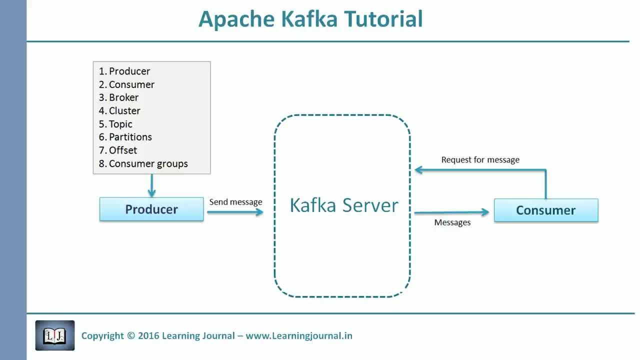 I will create a consumer application. Then I will request Kafka for the data. The Kafka server will send me some messages. I think you remember that each message is a line in this example. So the client application will receive some lines from Kafka server. 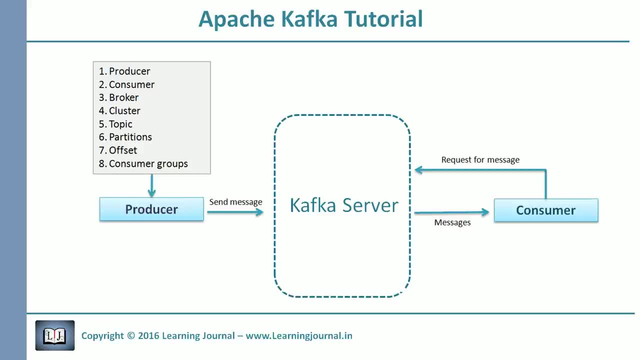 It will process them And again request for some more messages. The client keeps requesting data from Kafka And Kafka will keep giving message records as long as new messages are coming from the producer. Now let's move on and try to understand broker. The broker is a Kafka server. 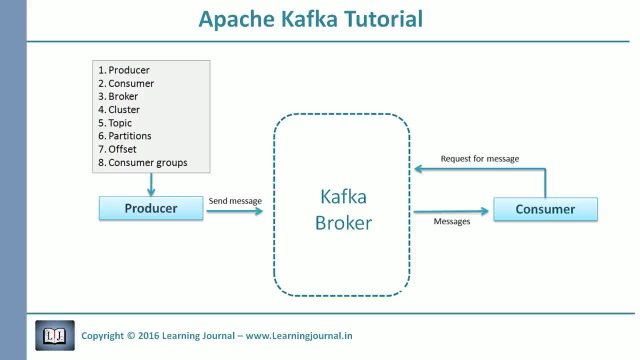 It's just a meaningful name given to Kafka server. And this name makes sense as well, because all that Kafka does is act as a message broker between producer and consumer. The producer and consumer don't interact directly. They use Kafka server as an agent or a broker to exchange messages. 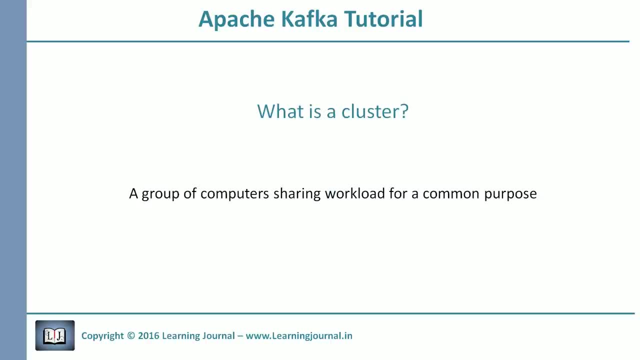 Ok, let's come to the next term, the cluster. This one is simple. If you have any background in distributed systems, you already know that a cluster is a group of computers acting together for a common purpose. Since Kafka is a distributed system, so the cluster has the same meaning for Kafka. 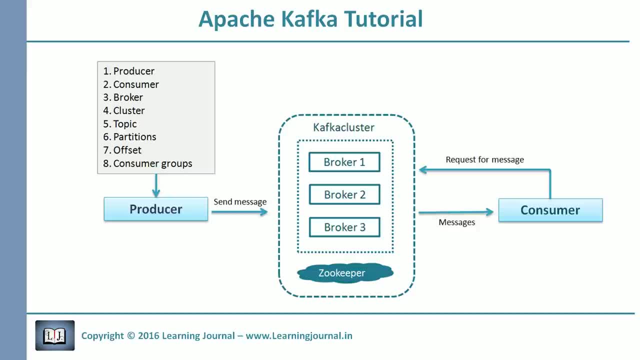 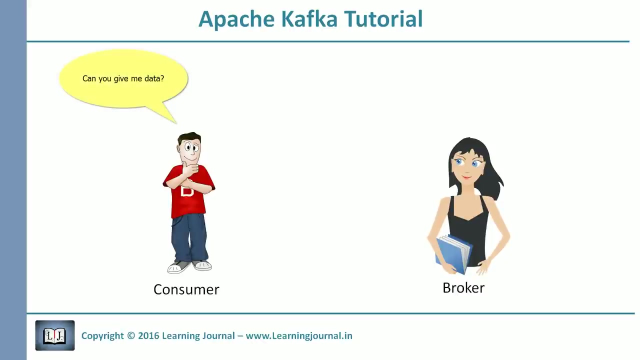 It is simply a group of computers each executing one instance of Kafka broker. Ok, the next item is the topic. We learned that producers send data to Kafka broker. Then consumers can ask for data. They collect data from the Kafka broker, But the question is, which data? 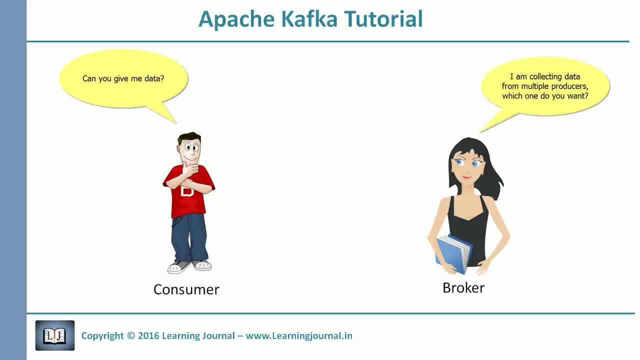 The broker says: Guys, I am collecting data from multiple producers. Which one do you want? Ok, give the data sent by producer ABC. Oh man, producer ABC is pushing three different types of records. Which one do you want? Ok, Well, send me the sales data. 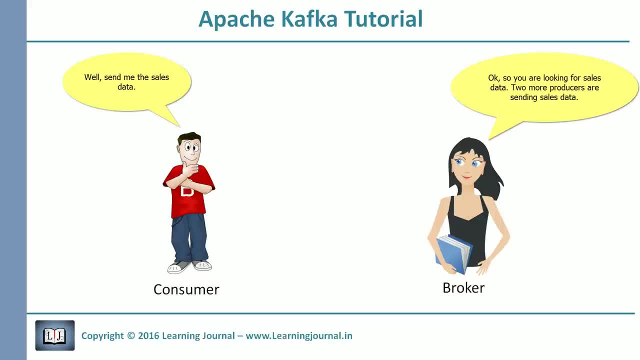 Ok, So you are looking for sales data. Two more producers are sending sales data. Gosh, we need to have some identification mechanism. There comes the idea of topic. So the topic is an arbitrary name given to a data set. We better say that it is a unique name for a data stream. 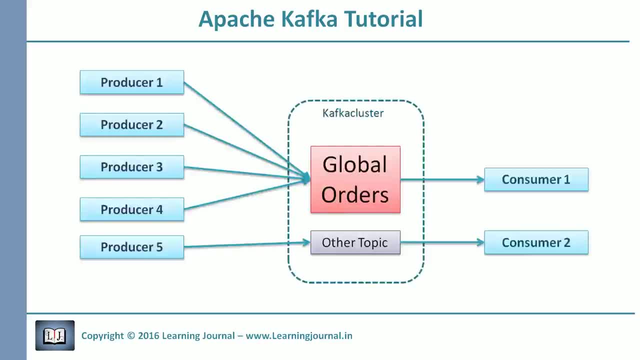 Ok, For example, we create a topic called global orders And every point of sale may have a producer. Each of them send their order details as a message to a single topic named global orders, And a subscriber interested in orders can subscribe to the same topic. 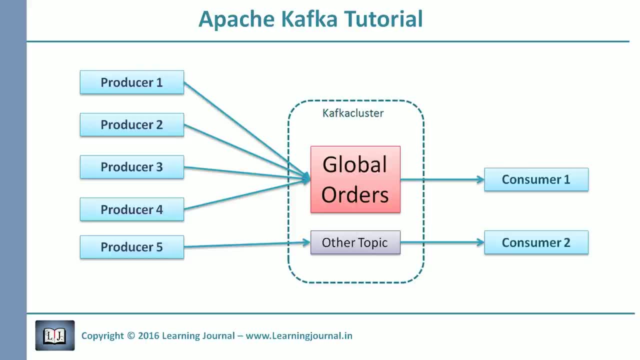 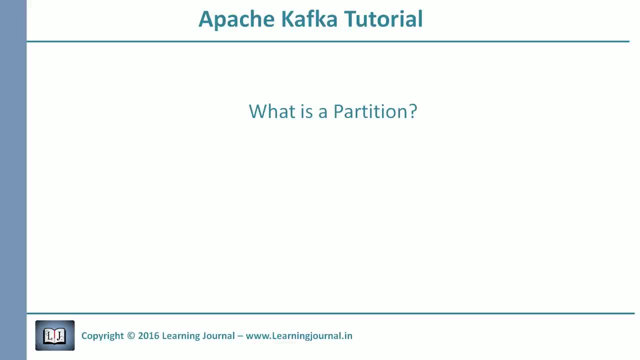 I guess You now have a fair idea about the topic. Let's come to the partitions. By now you learned that broker would store data for a topic. This data can be huge. It may be larger than the storage capacity of a single computer. 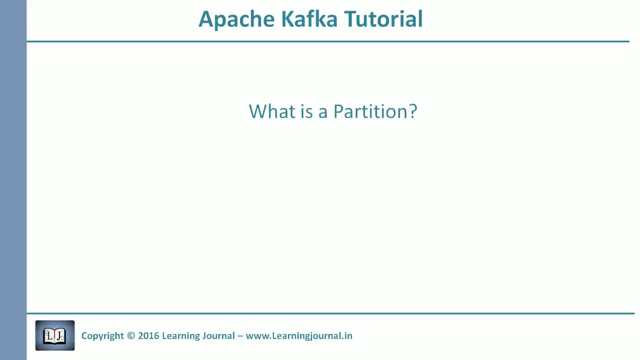 In that case, the broker may have a challenge in storing that data. One of the obvious solution is to break it into two. Ok, Ok, Let's write down two and break it into two or more total parts, 자� and distribute it to multiple computers. 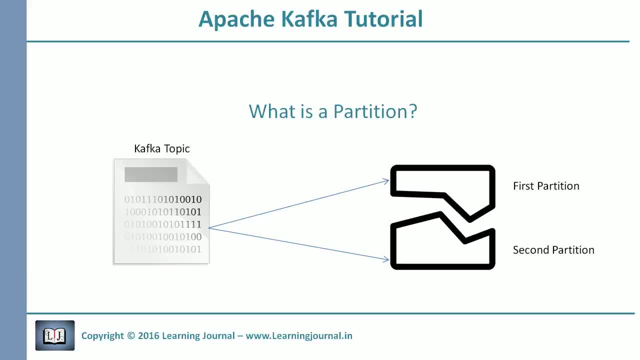 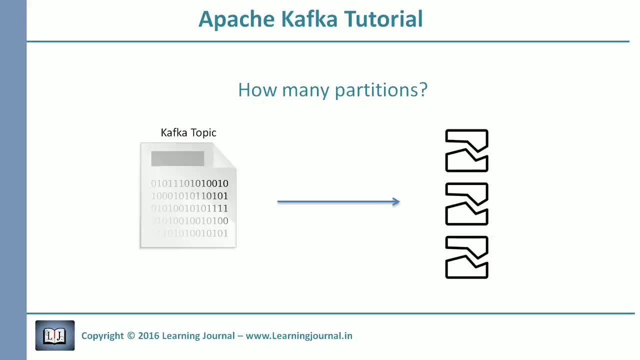 Kafka is a distributed system that runs on a cluster of computers. So it is very obvious that Kafka can break a topic into partitions and store one partition on one computer, And that's what the partition means. partitions, I mean some topic may be very large but others may be fairly small. So how Kafka knows. 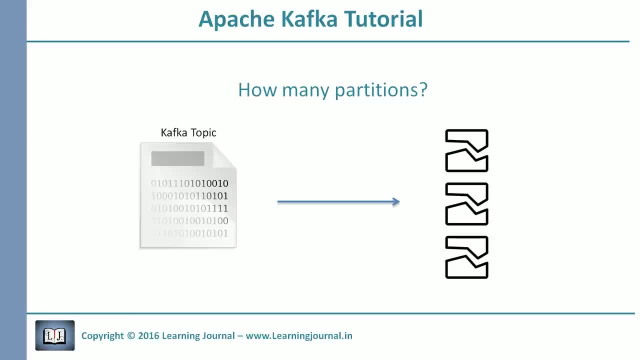 that it should create 100 partitions or just 10 partition should be enough. The answer is simple: Kafka doesn't take that decision. We have to take that decision. When we create a topic, we take that decision and Kafka broker will create that many partitions for your topic. 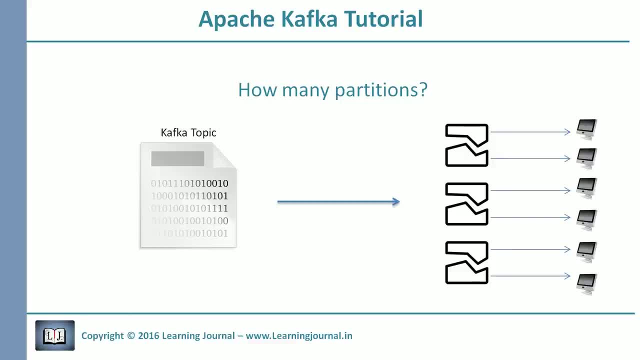 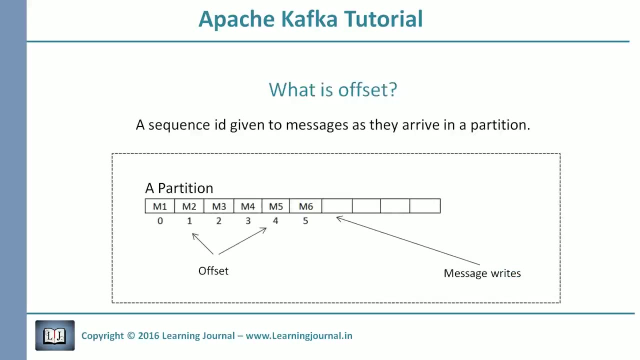 But remember that every partition sits on a single machine. You cannot break it again. So do some estimation and simple math to calculate the number of partitions. I think you know partitions now. Now let's talk about offset. The offset is simple. It is a sequence number of a message in a partition. This number is assigned as: 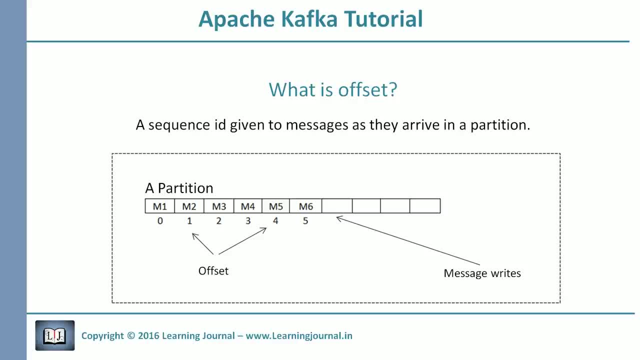 the number of partitions in the message. So let's take a look at the number of partitions. Let's take a look at the number of partitions in the message. So let's take a look at the number of partitions in the message. the message arrives in the partition And these numbers, once assigned. 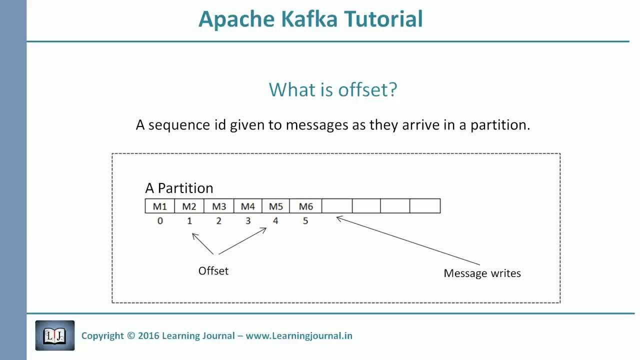 they never change, They are immutable. The sequencing means that Kafka stores messages in the order of arrival. within a partition, The first message gets an offset zero, The next message gets an offset one, and so on. But remember that there is no global offset. 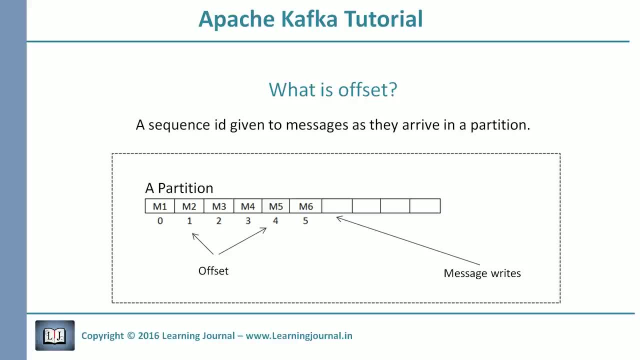 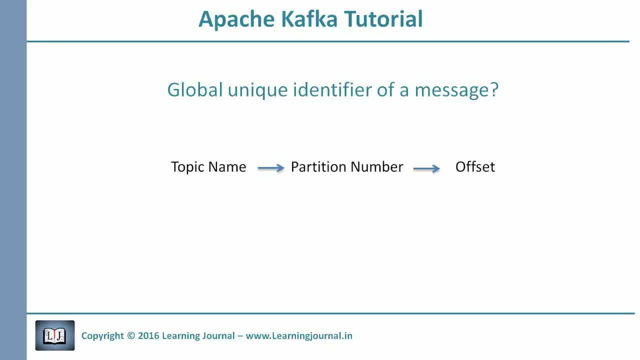 across partitions, Offsets are local to the partition. So if you want to locate a message, you should know three things: Topic name, partition number and offset number. If you have these three things, you can directly locate a message. Now we are left with the. 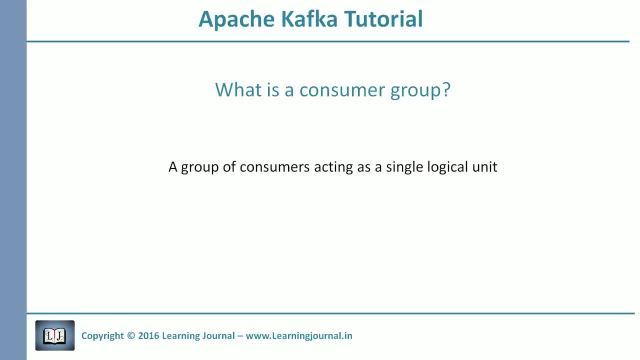 last thing, The consumer group. So we already understand the consumer. What is a consumer group? It is a group of consumers. So many consumers form a group to share the work. You can think of it like there is one large task and you want to divide it among multiple. 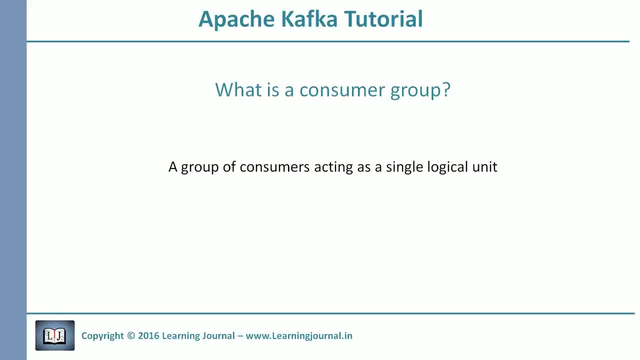 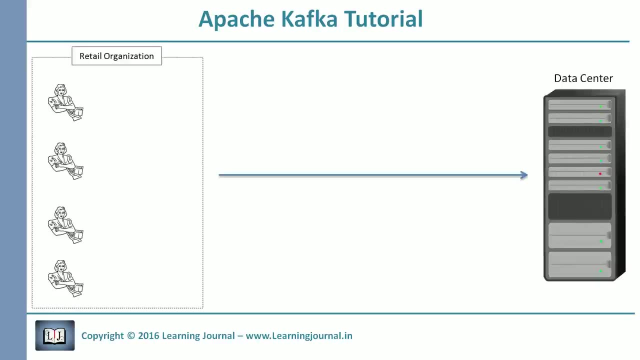 people, So you create a group and members of the same group share the work. Let me give you an example. Let's assume that we have a retail chain. In every store there are few billing counters. You want to bring all of the invoices from every billing. 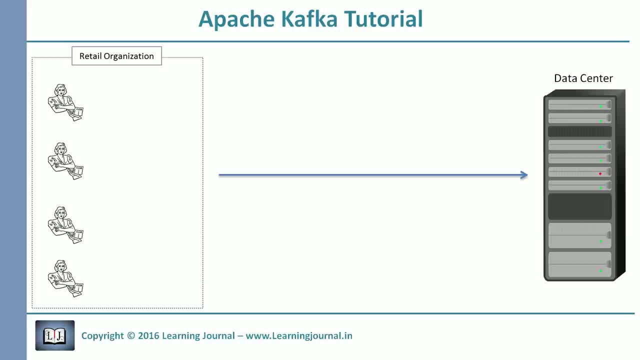 counter to your data center. Since you learned Kafka and you find Kafka as a good solution to transport data from billing locations to the data center, you decided to implement it. The first thing you might want to do is to create a producer at every billing location. 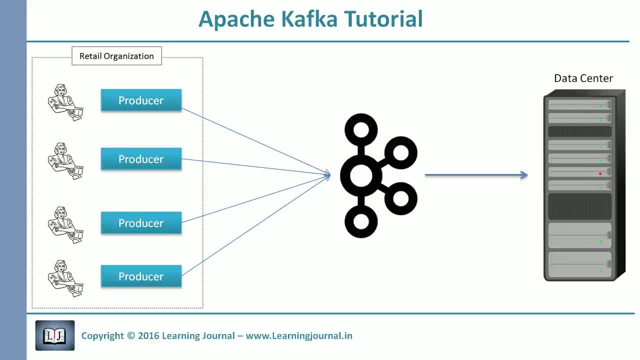 These producers will send bills as a message to Kafka topic. The next thing you might want to do is to create a consumer. The consumer will read data from Kafka topic and write them into your data center. It sounds like a perfect solution, right? But there is a